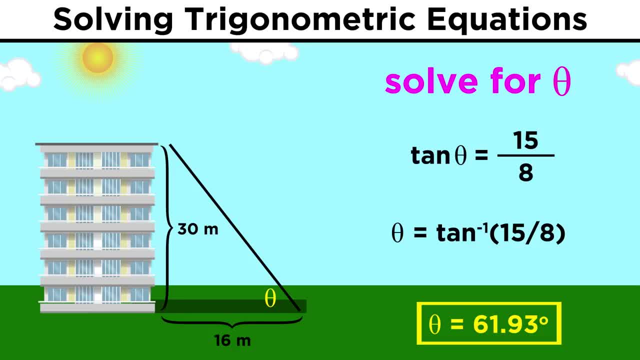 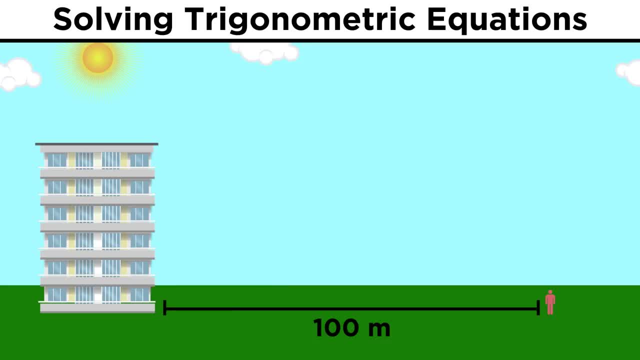 get just a hair under 62 degrees. We can do all kinds of useful things of this nature using trig functions. If we know how far away some building is, we can instantly know how tall it is, just by measuring the angle of elevation required for u-dimensional trigonometry. 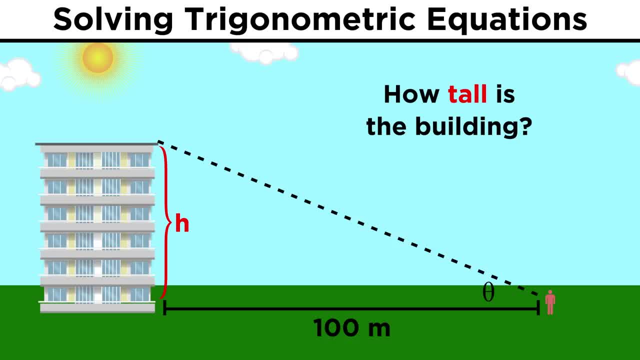 Thanks for watching your line of sight. to coincide with the top of the building. If this distance is 100 meters and this angle is 55.3 degrees, then we can take the tangent of the angle, which will be equal to this height over 100, then multiply by a hundred. 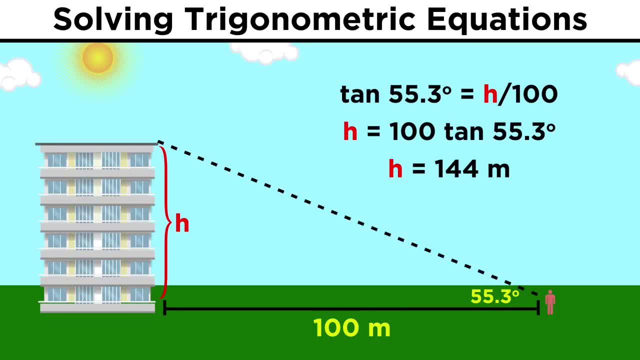 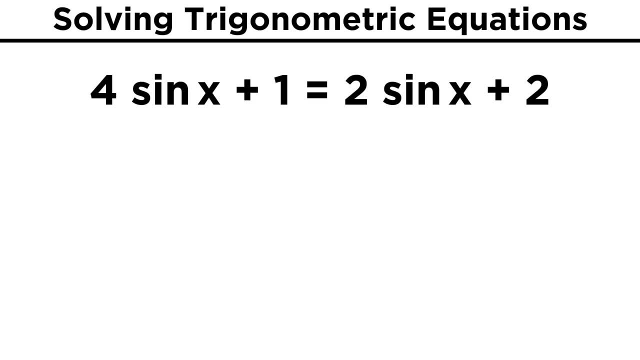 and we get around 144 meters. So these are indeed powerful techniques, But beyond this, we need to be able to solve trigonometric equations, meaning we need to be able to look at equations with trig functions in them and solve for X. 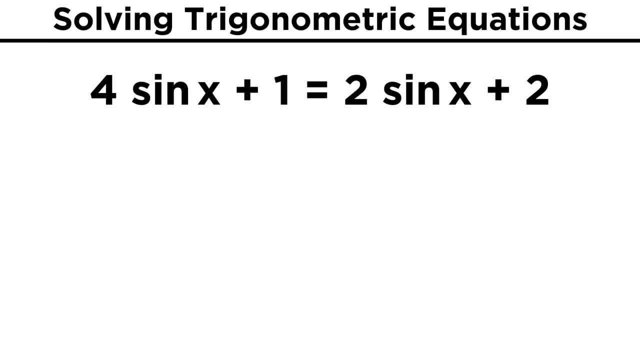 Say we have four. sine X plus one equals two. sine X plus two. First we need to combine like terms. so let's subtract two sine X as well as one, That gives us two. sine X equals one Divide by two and sine X equals one. 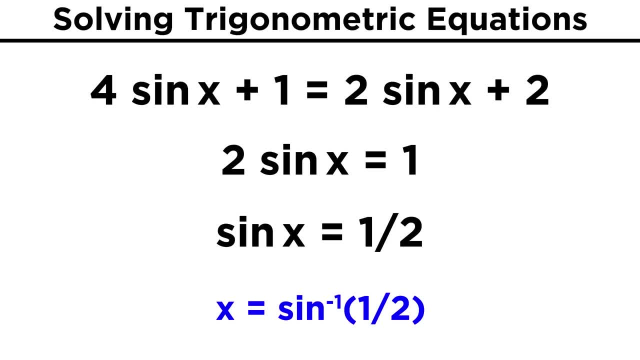 That equals one half. Now to solve for X, we can definitely take the inverse sine of one half, or we can picture the unit circle and recall that pi over six has a sine value of one half. But the only problem is that this is not the only solution to this equation. 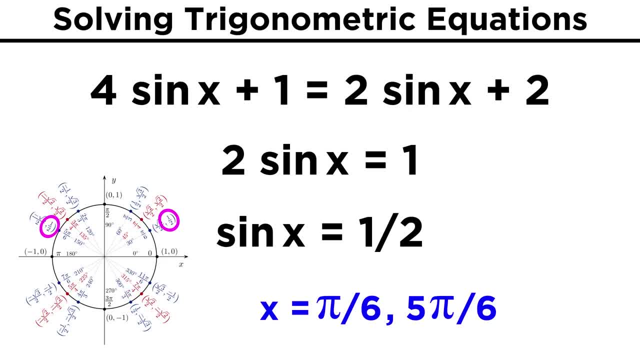 The sine of five sixths pi also gives one half. Not only that, but either of these values plus any multiple of two pi will also give one half. This will also be a solution because, starting at one sixth pi, if we go all the way around, 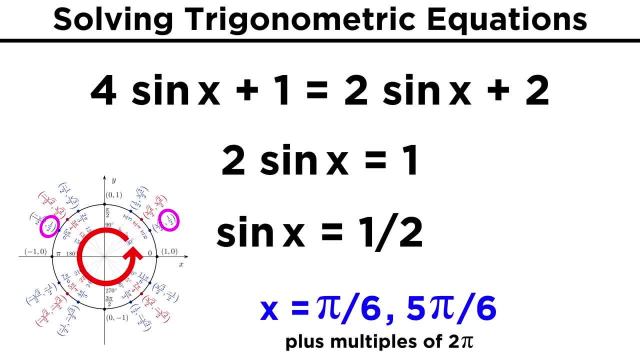 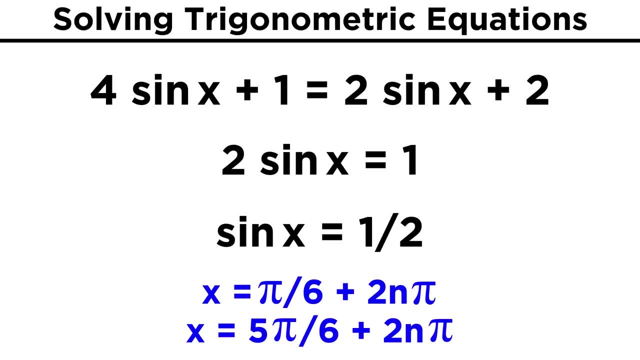 to get here again, which would be thirteen sixths pi. that will also be a solution. Therefore, the way we express this solution will be one sixth pi plus two n pi and five sixths pi plus two n pi. With these n can be any integer, so if it's one, this is two pi. 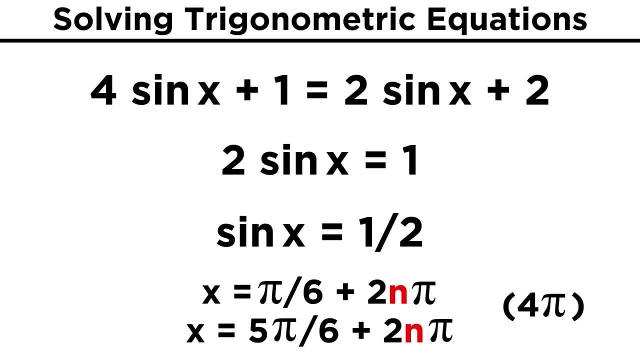 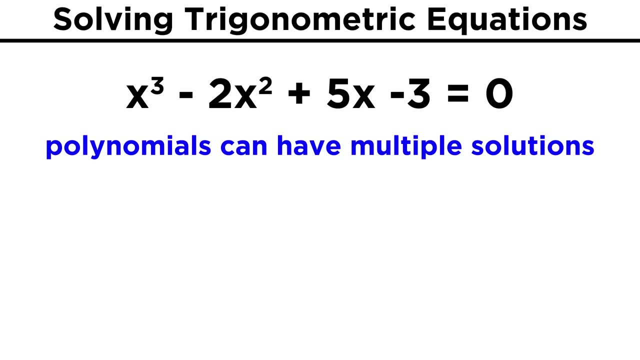 If it's two, we get four pi. Whatever it is, it represents some number of times going around the unit circle to get back to the same spot and therefore another solution to the equation. In this way, just as algebraic equations often have zero, one or multiple solutions, trigonometric 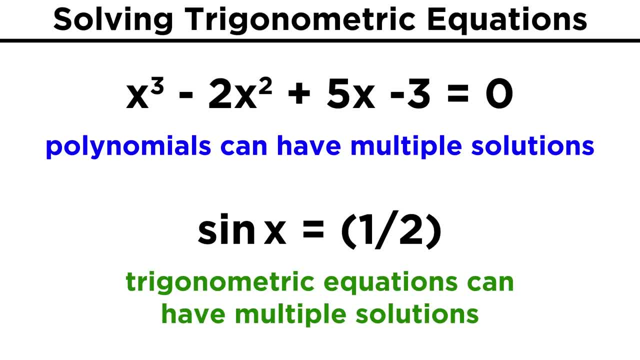 equations often have multiple or even infinitely many solutions. Things get a little more complicated when we start manipulating the above and below. Try a little bit of rhythm and you'll get a equivalent of the two pi you didn't take manipulating the trig functions. 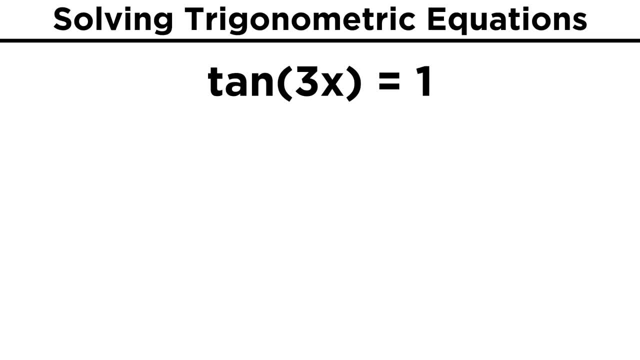 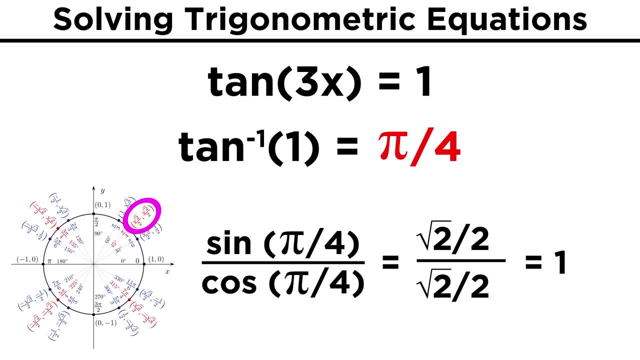 Say we want to solve tangent: three X equals one. Well, what angle gives us a tangent of one? That would be quarter pi, because root two over two, divided by root two over two, gives us one. That means that three X equals quarter pi. 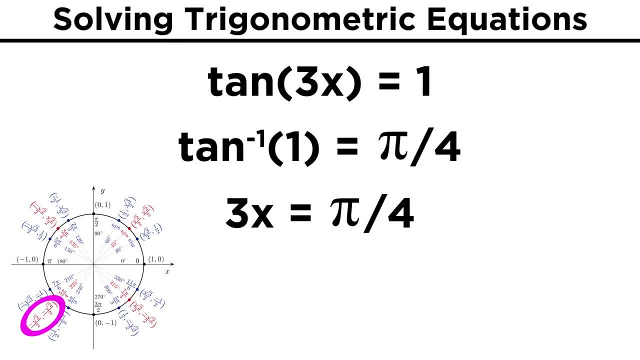 But is it just quarter pi? If we go to the other side, negative root two over two divided by negative root two over two also gives us one for the tangent. so five fourths pi works as well. That means that three X equals quarter pi plus N pi. 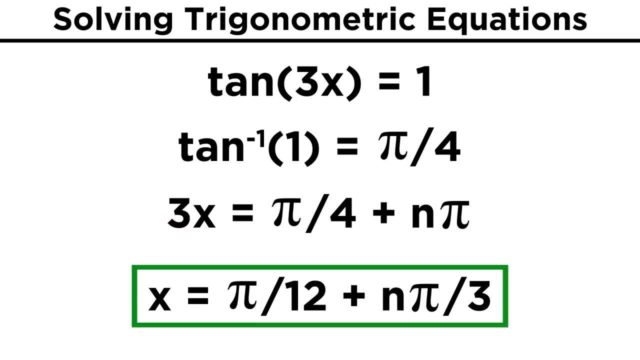 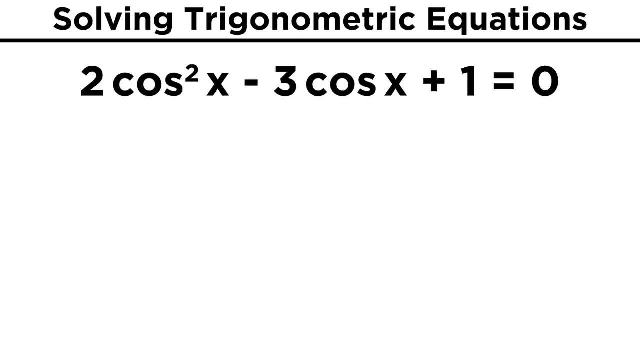 Now to solve for X, we divide both sides by three. That leaves us with pi over twelve plus N, pi over three. Trigonometric equations get much more complicated. We can even see them in quadratic form. Take something like: two cosine squared, X minus three. cosine X plus one equals zero, and we: 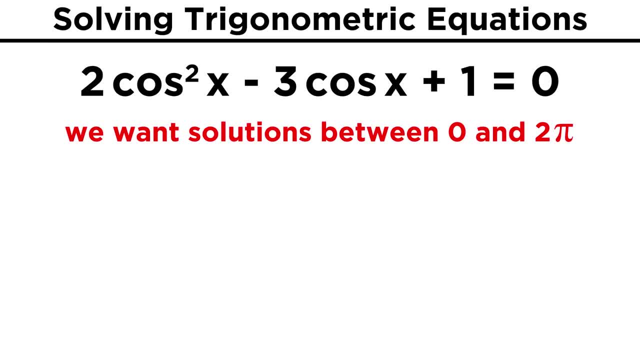 are just looking for answers in the interval from zero to two pi. It may look different than your typical polynomial, but we can factor this into binomials just like we normally would. We know we will need two: cosine X here and cosine X here. 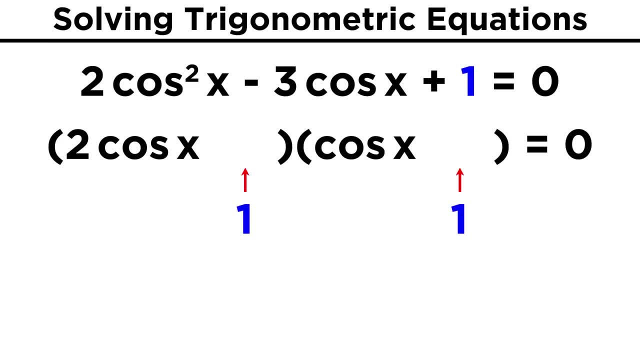 Then from there, we'll need two: cosine X here and cosine X here. From there, the factors of one are either one and one, or negative one and negative one. Since this cosine term is negative, let's try the negatives, and that does indeed work. 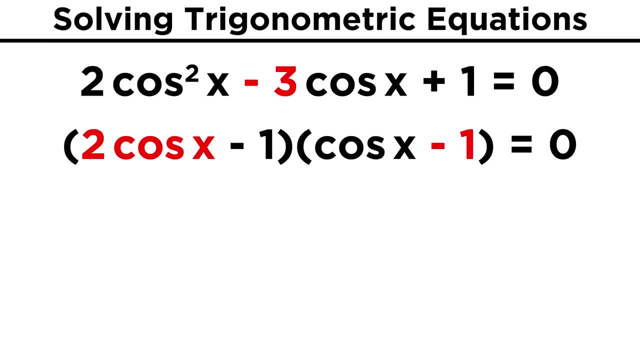 out, since we get minus one cosine here and minus two cosine there. Now, as we know, each of these binomials can be set equal to zero, giving us two cosine X equals one, or cosine X equals one half, and then cosine X equals one. 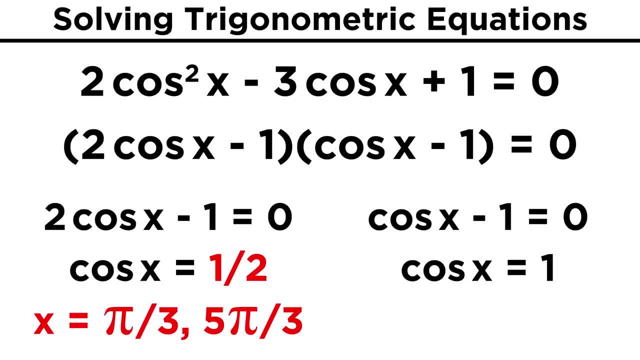 Well, where does cosine equal one half? That would be at one third pi and five thirds pi. Where does cosine equal one At zero? So the solutions are zero, one third pi and five thirds pi. There are other situations where we will have to factor in a different way. 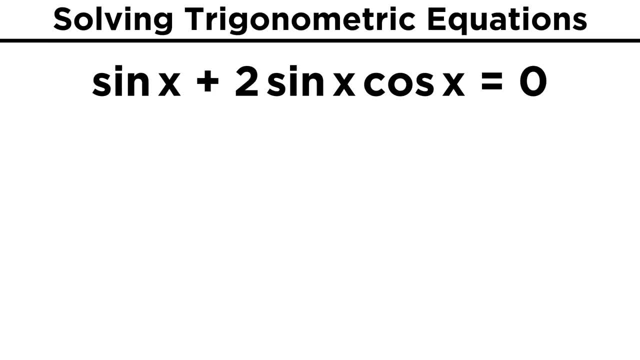 Take sine X plus two sine X cosine X, solving for the interval from zero to two pi. These two terms are equal and the answer is zero. These two terms have sine X in common, so let's factor it out. That leaves us with sine X times the quantity one plus two cosine X. 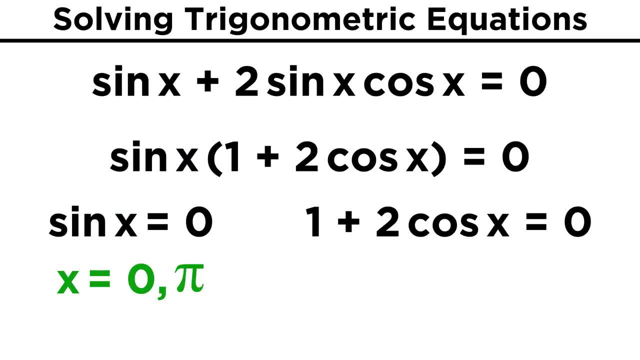 Now, if sine X is zero, this whole side is zero. so zero and pi are solutions, because the sine of zero and the sine of pi both equal zero. Then for this one two cosine X equals negative one and cosine X equals negative one half. 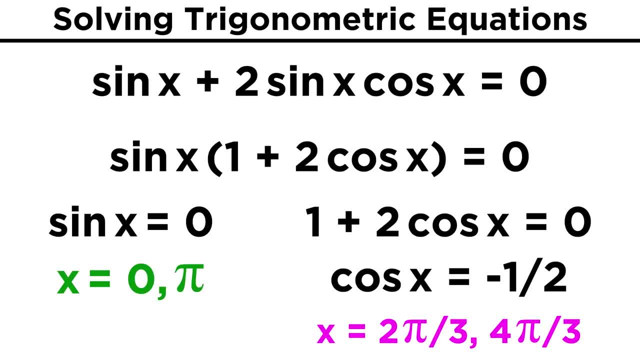 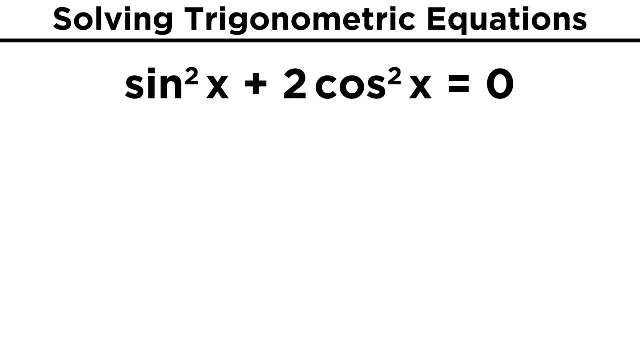 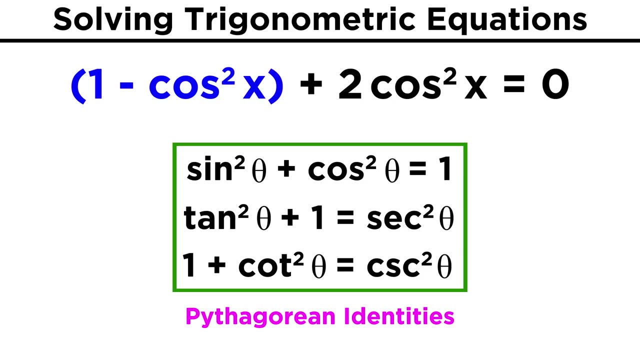 That means that two thirds pi and four thirds pi are also solutions. Other strategies involve using trigonometric identities. If we have an expression with sine squared terms and cosine squared terms, we can change one of them to the other using this identity. There are too many identities to do examples for each and, as we have already learned, the 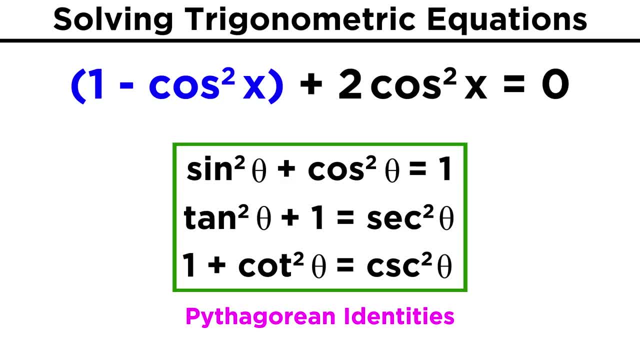 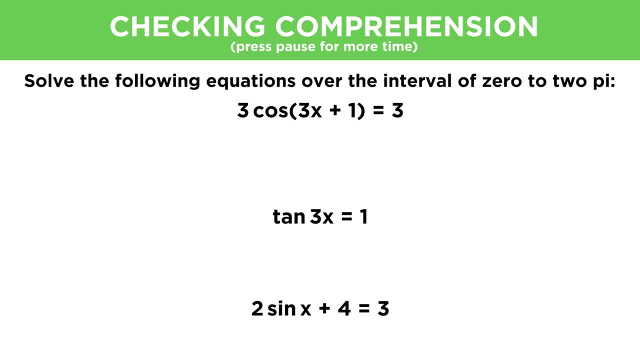 identities just remind ourselves that all of these strategies are at our disposal. I think we get the idea, so let's check comprehension. Thanks for watching, guys. Subscribe to my channel for more tutorials. support me on Patreon so I can keep making. 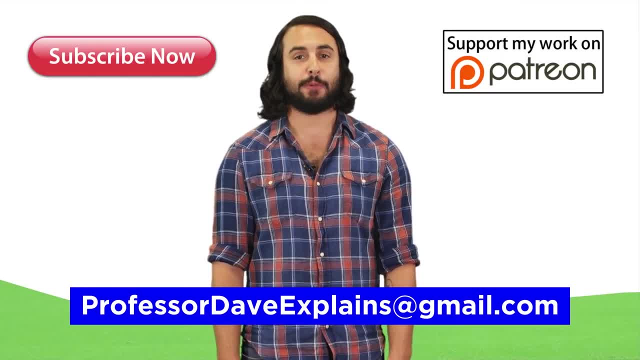 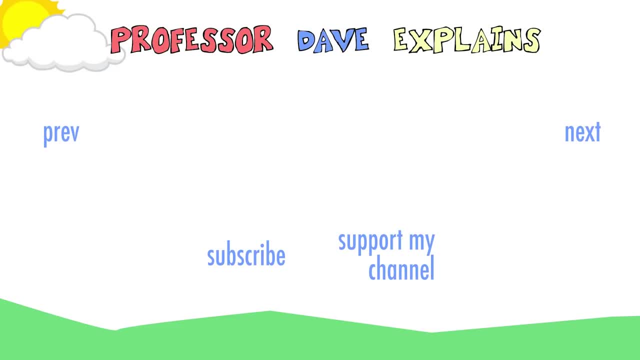 content and, as always, feel free to email me professordaveexplains at gmailcom. I'll see you next time.